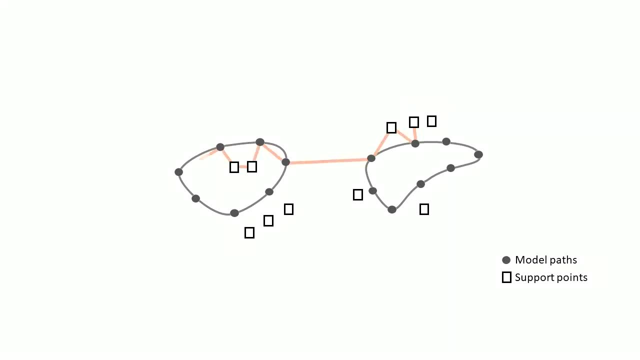 the support points Using a shortest Hamiltonian path algorithm. on this set of points, we can then compute a continuous path that passes through all the model points and all the support points. The resulting path will generally not follow the model path continuously, which leads to: 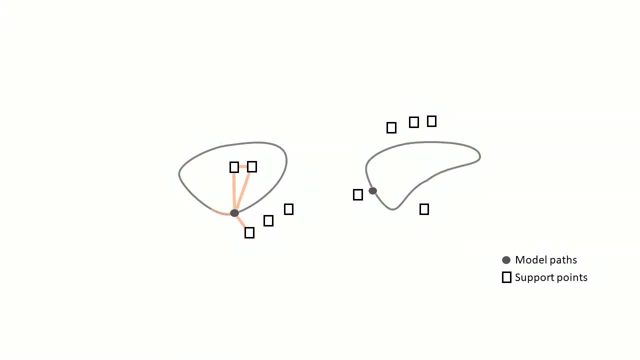 unacceptable print quality. To avoid this problem, we represent model paths using a single connection point that we pass to the shortest path. solver. The resulting path allows us to branch out at connection points and print the cyclic model path as one continuous segment. However, the generated path still crosses the model multiple times, which would lead. 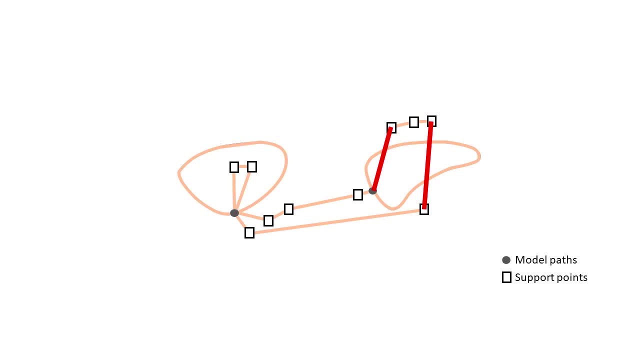 to unacceptable artifacts once printed. We address this problem by modifying the model path as a continuous segment. We then create a continuous path that passes through all the model points and all the support points. We then create a continuous path that passes through all the model points and all the support points. 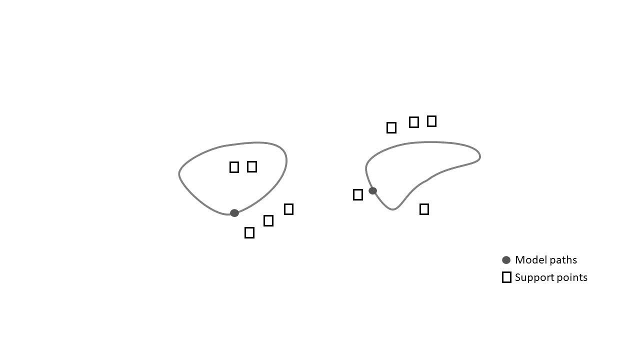 We then create a continuous path that passes through all the model points and all the support points. We thenati the cost of model crossing path segments to reflect the length of a corresponding model avoiding path. To this end, we first introduce safeguarding proxy geometry around the model path, allowing 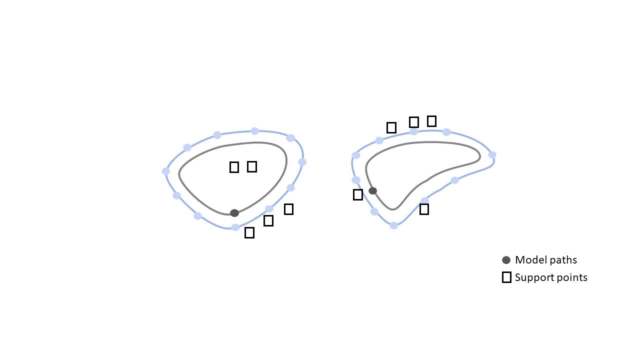 the deposition path to navigate around the model at a close but safe distance. We then construct a graph containing the proxy geometry and all support points, but discard other edges that cross through the model. Using Dijkstra's algorithm, we then compute all pairwise distances between the points. 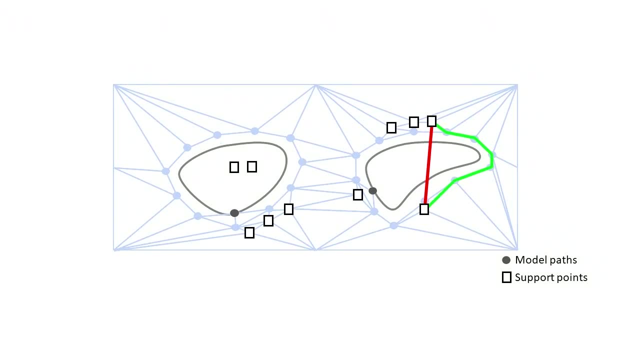 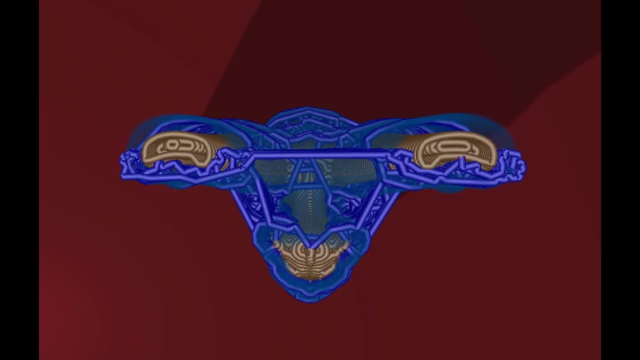 of the graph and pass the corresponding model avoiding metric through the shortest Hamiltonian Hamiltonian path algorithm. The resulting path allows us to print all model paths continuously without crossing through the model unnecessarily. Applying our path planning algorithm from top to bottom in each layer yields a single. 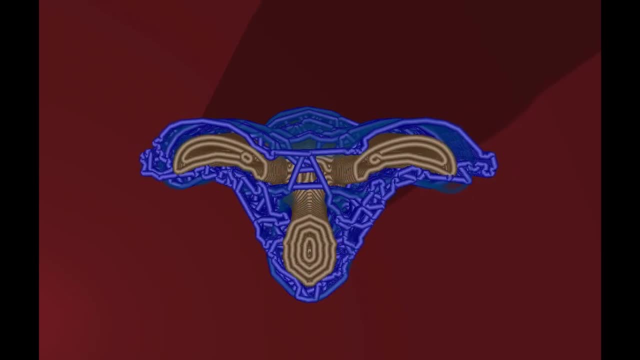 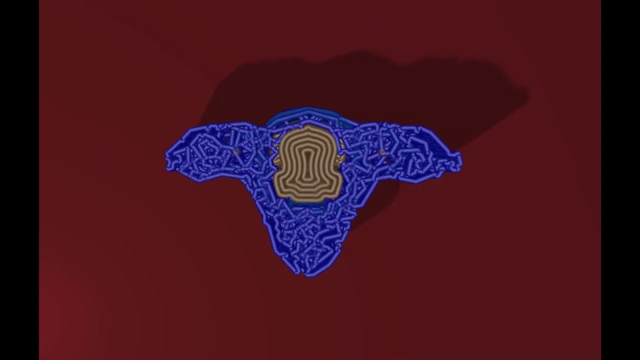 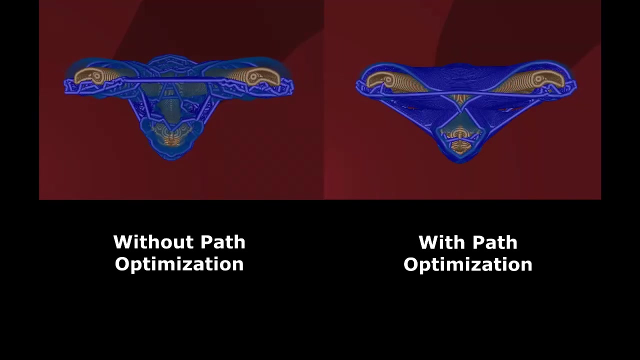 continuous self-supporting deposition path. Without modification, however, the generated path would grow in length and complexity from top to bottom, increasing print time, material cost and the difficulty of removing the non-model structure. We solved these issues by optimizing the shape of the non-model structure with respect to 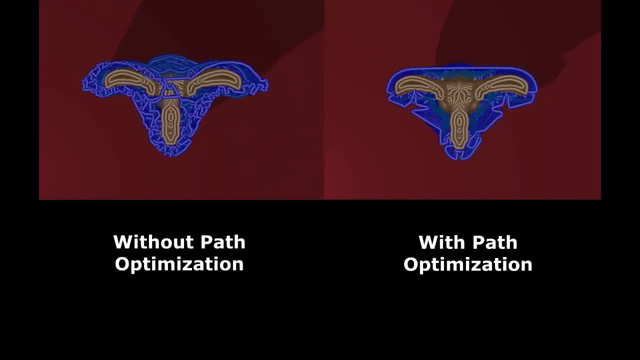 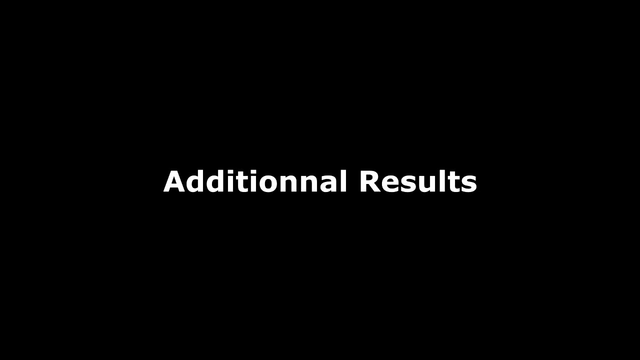 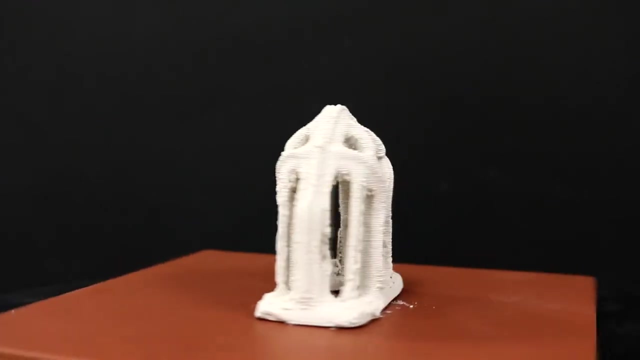 length, curvature and distance to the model. As can be seen in this comparison, path optimization leads to significantly smoother and less dense non-model structure that is faster to print and easier to remove. Please refer to the paper for more details. Thank you for watching.